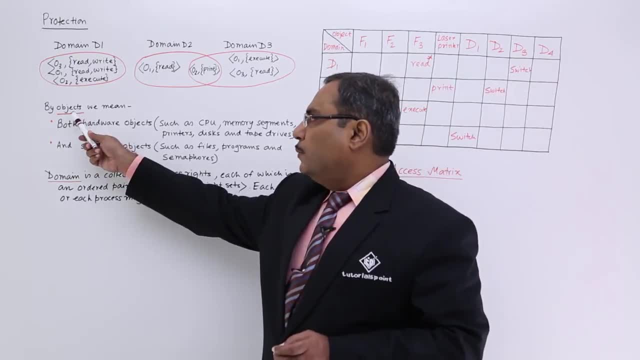 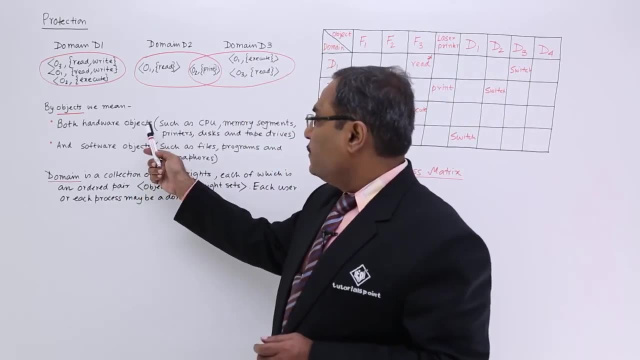 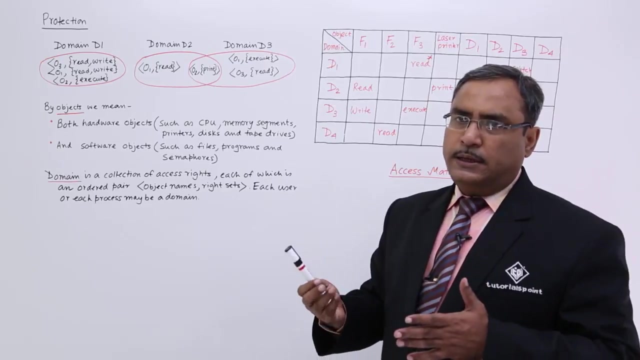 diagram for further explanation. By objects we mean the hardware objects or the software objects, So it can be hardware or software. In case of hardware objects such as CPU, memory segments, printer disks, tape drives, it can be one object. that means some hardware. 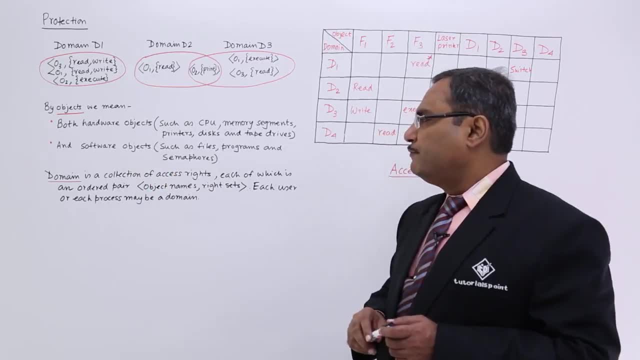 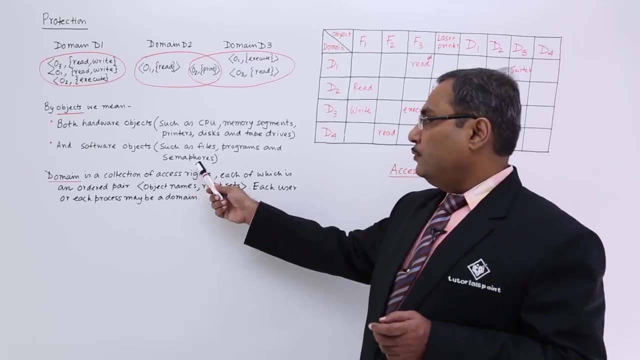 resources. In case of software objects, we can go for a files, we can go for programs, we can go for semaphore. Semaphore is a synchronization tool, So semaphore, and these things will be known as the software objects, So objects. we have got the idea. 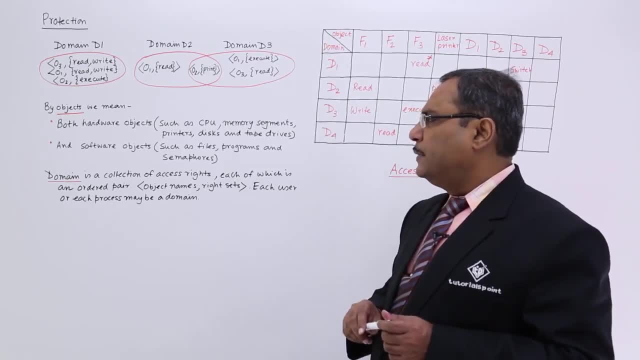 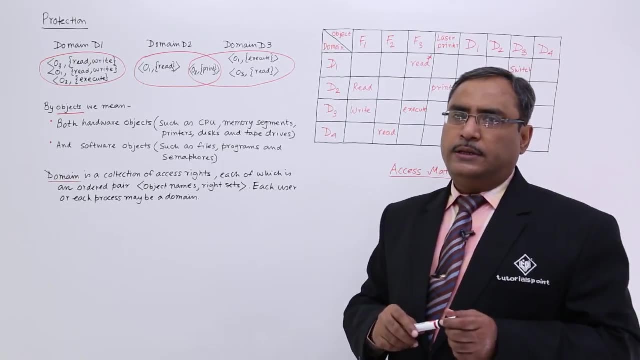 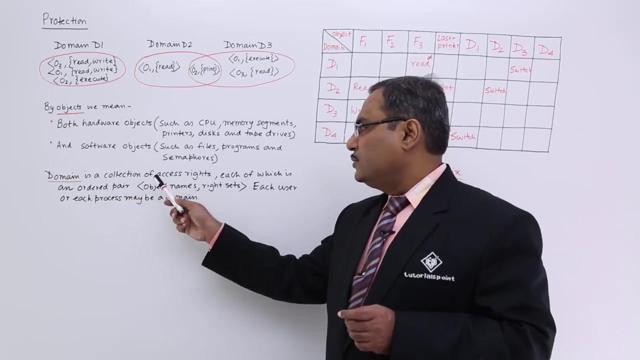 Now let us go for the domain. Domain is nothing but a collection of access rights. What are the access rights? Access rights may be, say read access right, say write access right, or say your execute access right. So is a collection of access rights, each of which. 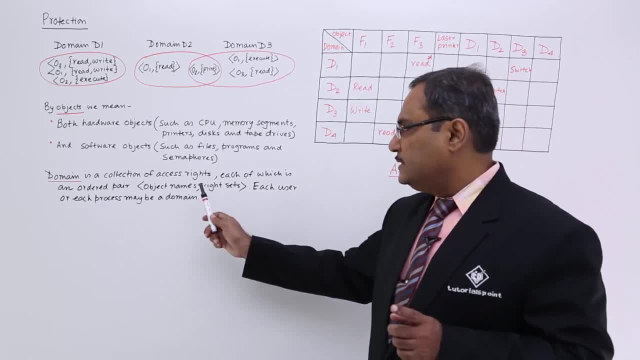 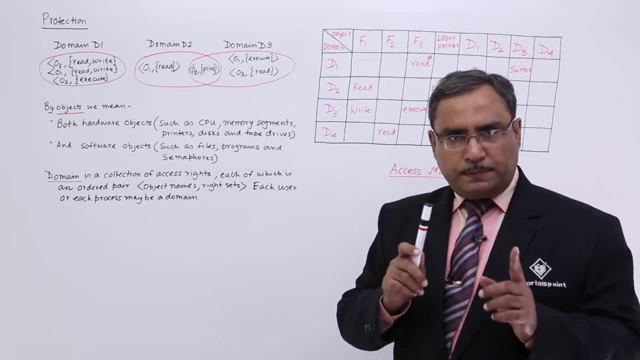 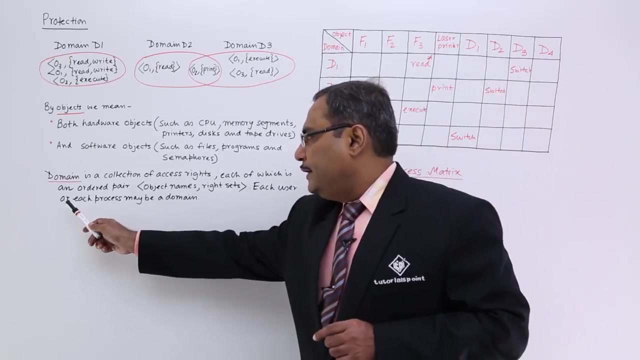 is an ordered pair. Ordered pair means this sequence has to be maintained. At first object names will be coming, then write sets will be coming. So the ordered pair means this ordering has to be maintained. You cannot write on the other way. Each user or each process may be a domain, So each user can be treated as 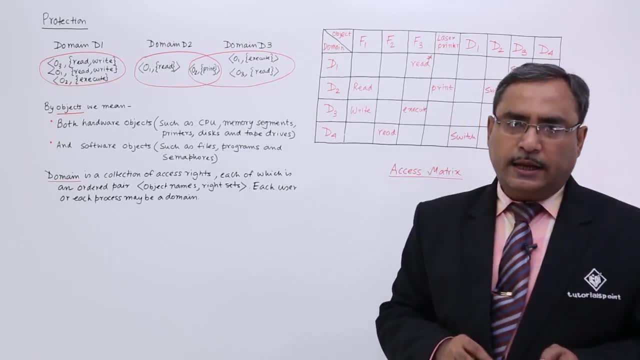 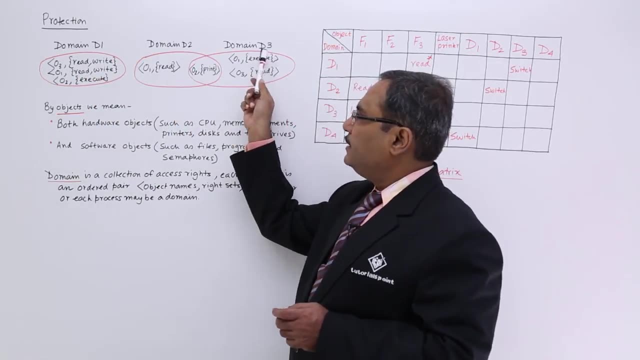 one domain or each process may be treated as a domain. Now, you see, this is the domain Let us call. the name is D 1,, this is D 2,, this is D 3.. And you see, we are having this object and access rights as a paired, ordered pair On. 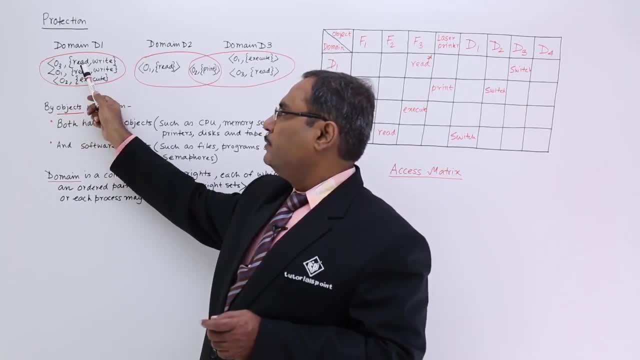 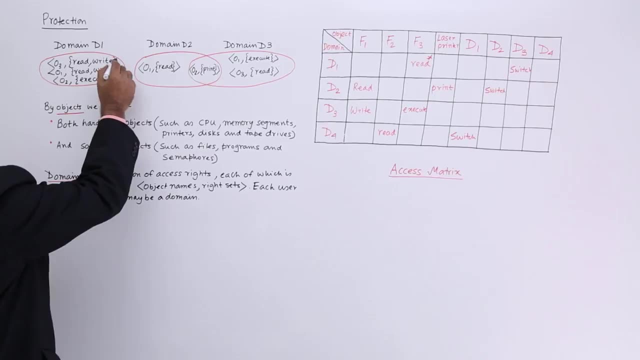 this particular object- O 3, read write can be performed. O 1, read write can be performed. O 2, only the execute can be performed, And similarly for this one. So this is known as the domain. This is known as the domain And in this particular case also, we are having 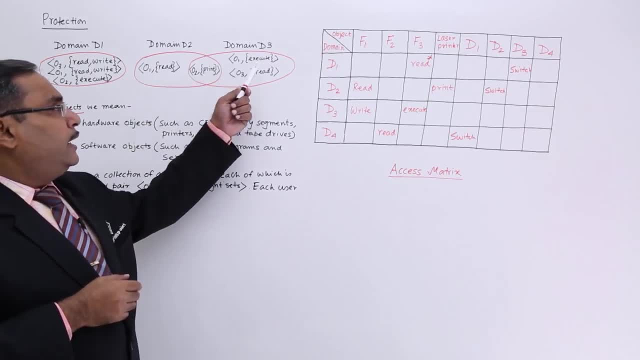 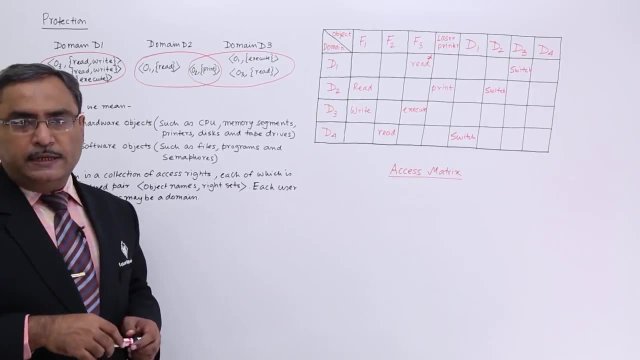 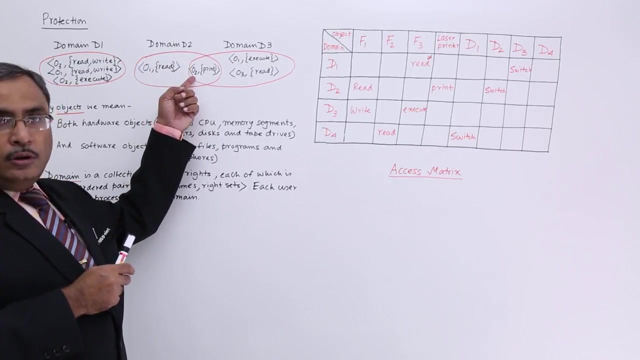 this object 1, where read operation can be performed, and these other things are there. This is object to print- is common between D 2 and D 3.. That means if one user finds himself or herself in this particular D 2, can also go for object to print And another.